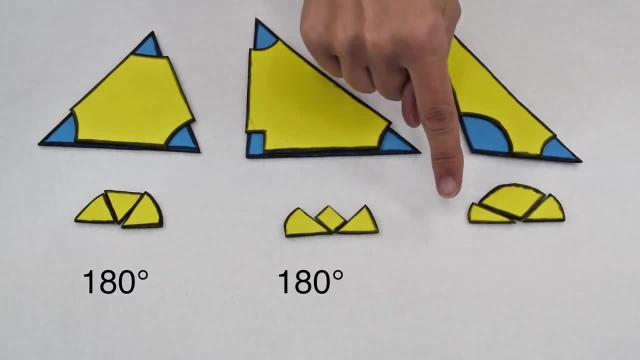 and arrange them, we see that they also go together to form a straight line. That means all triangles are going to have an interior angle sum of 180 degrees, regardless if they're regular or irregular. Let's look at a few other irregular polygons, Starting at one vertex. we're going to 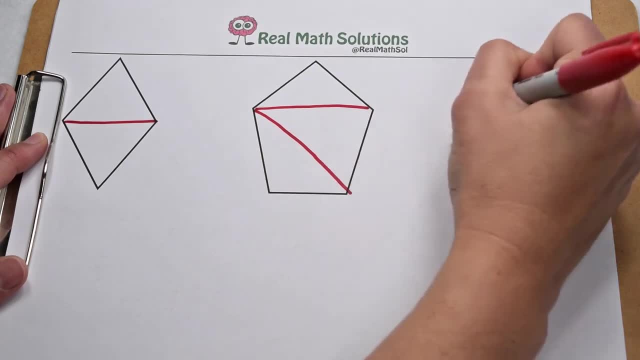 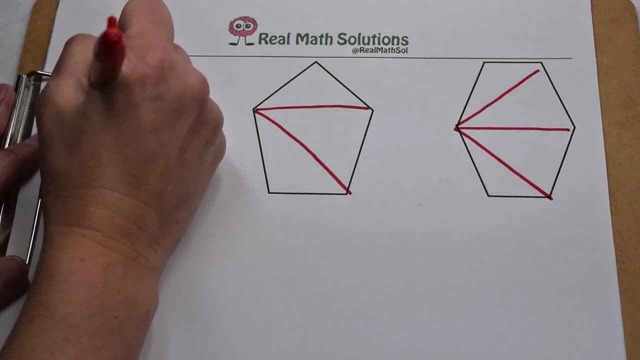 connect that vertex to all the other vertices in our figure. When we do that, we create a set of triangles. We know that each triangle has an interior angle sum of 180 degrees, so we're going to use that to help us find the interior angle sum of 180 degrees. We're going to use that to help us. 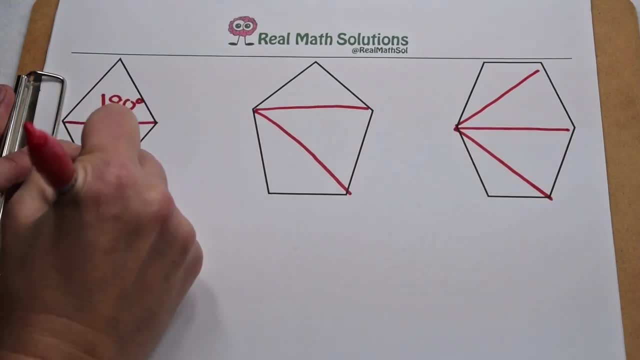 find the interior angle sum of the entire figure. Here on the quadrilateral we've made two triangles. We know each triangle is worth 180 degrees. So 180 degrees times 2 is going to give me an interior angle sum of 360 degrees on the quadrilateral. Same thing on the pentagon We. 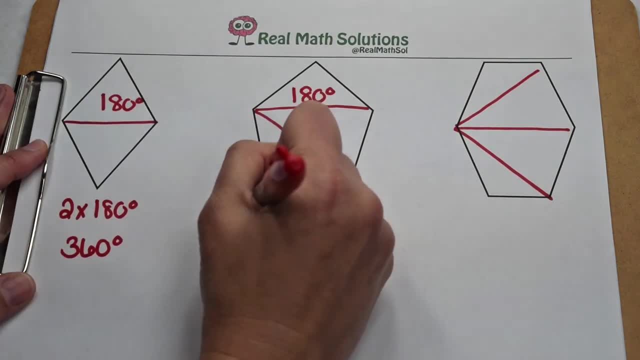 know that each triangle is worth 180 degrees and we created three triangles. So to find the interior angle sum, I'm going to multiply 3 times 180, and that gives me 540 degrees. Here on the hexagon, each triangle is worth 180 degrees. So I'm going to multiply 3 times 180, and that gives me: 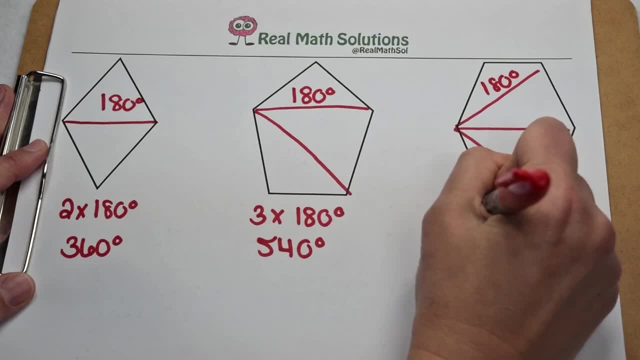 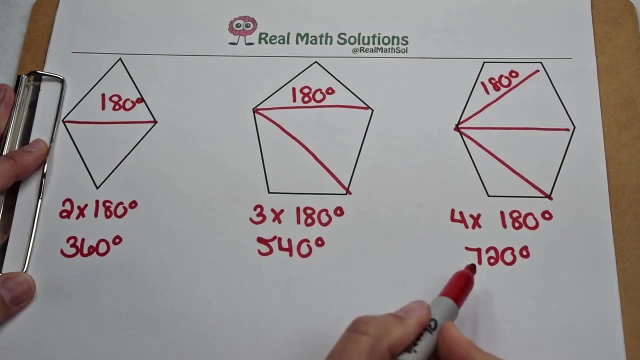 180 degrees and we've made four of them. So to find the interior angle sum I'm going to multiply four times 180.. Four times 180 gives me an interior angle sum on the hexagon of 720 degrees. Let's take our data, arrange it in a table so we can look for a pattern. 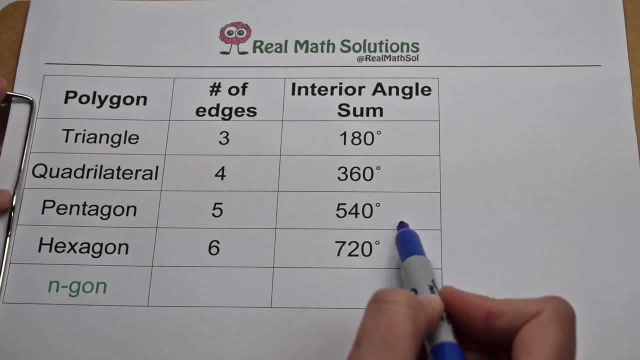 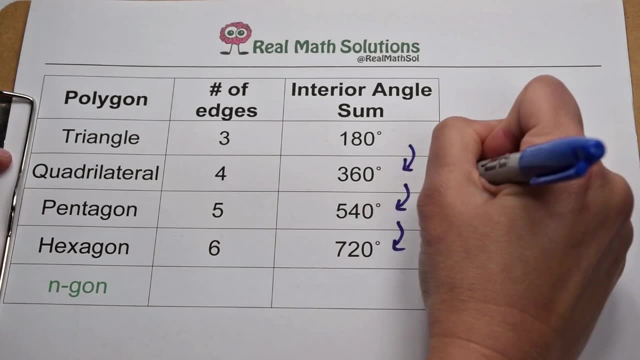 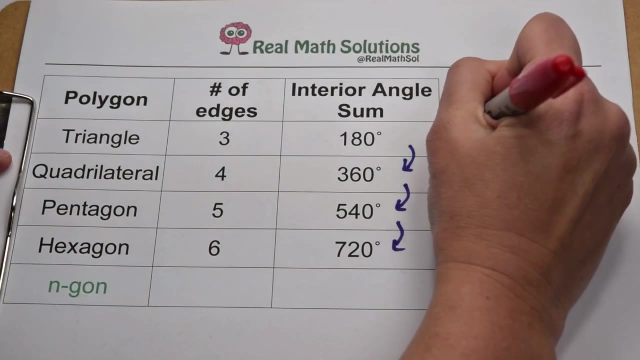 Triangles, no matter what, are 180, quadrilaterals 360, pentagons 540, hexagons 720.. Well, if we look, we can again see that we are constantly increasing by 180 degrees each time. So that means we're again working with multiples of 180.. So the triangle would be 1 times 180,. 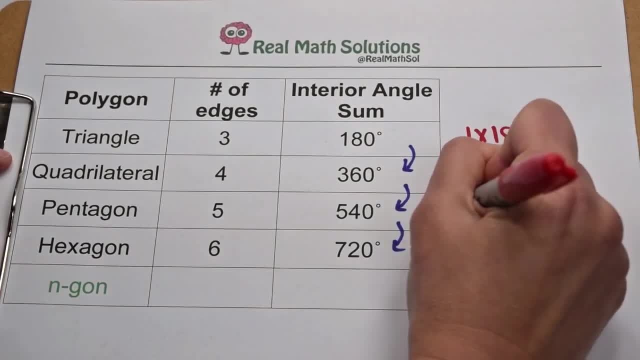 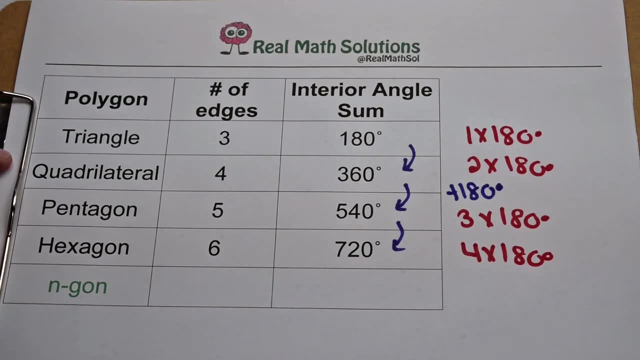 the quadrilateral is still 2 times 180, the pentagon 3 times 180, and our hexagon is 4 times 180. So, just like with regular polygons, we can see that we're always multiplying something times 180.. So if we want to generate that in an equation for our n-gon meaning any, 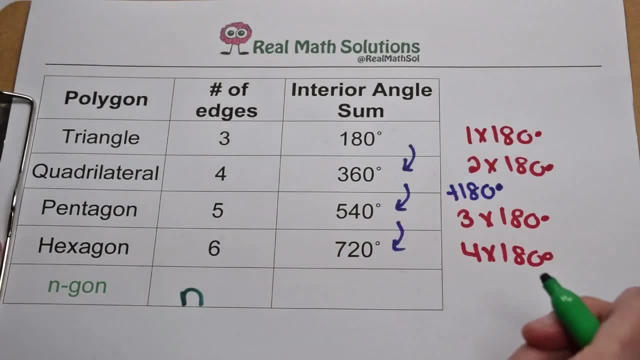 number of sides. we know we're going to multiply something times 180.. Well, again, if we look, the triangle would be 180 degrees and the hexagon would be 4 times 180.. So if we want to generate that in an equation for our n-gon, meaning any number of sides, we know we're.